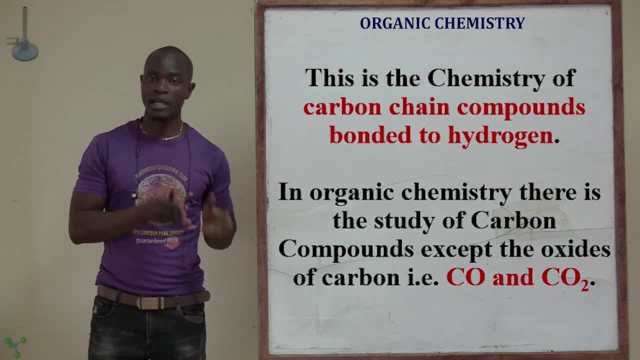 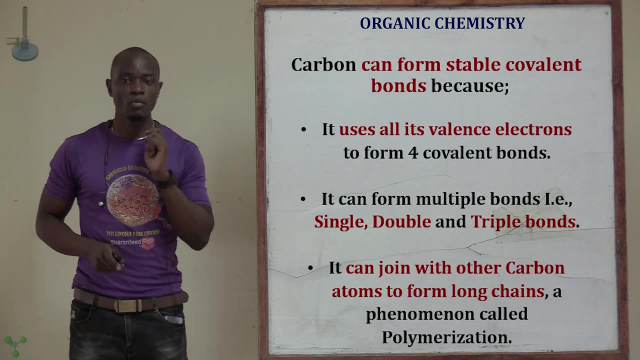 chemistry is study the carbon chain compounds bonded to hydrogen, as well as other atoms that you are going to look at, but not carbon oxygen compounds comprising of carbon two oxide and carbon four oxide compounds. so you see that the carbon element can be able to form stable covalent bonds with other carbon atoms and with other elements, because we see that 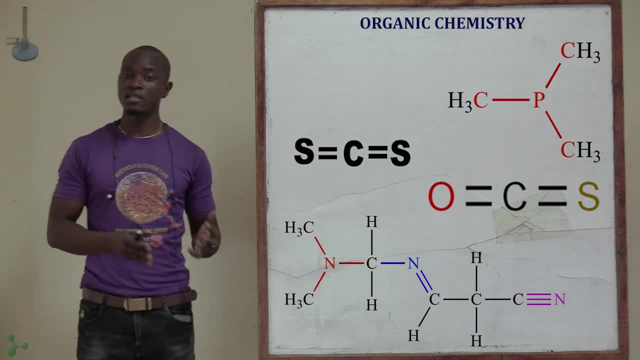 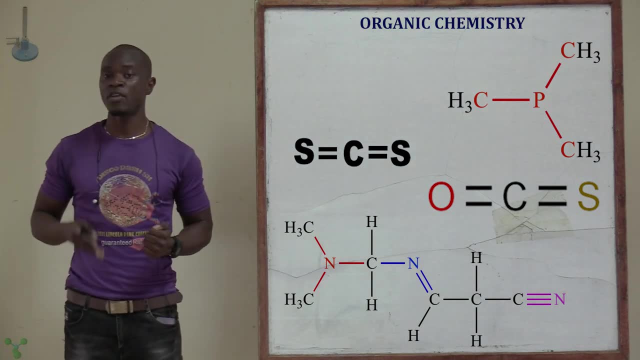 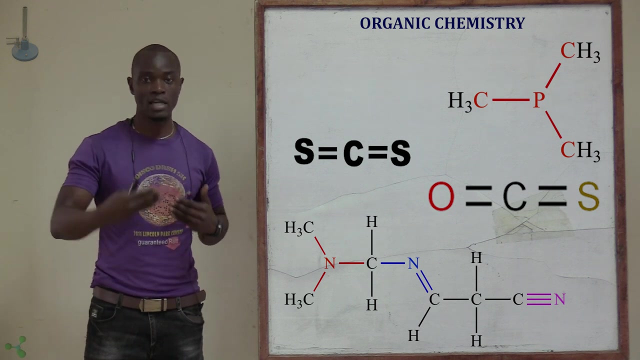 in these chains that we have in organic chemistry, we can see that this carbon atom is able to bond to other carbon atoms as well. it is able to bond to other different types of atoms that we have. it's not only carbon bonding with hydrogen, but can the carbon can bond with other carbon atoms. 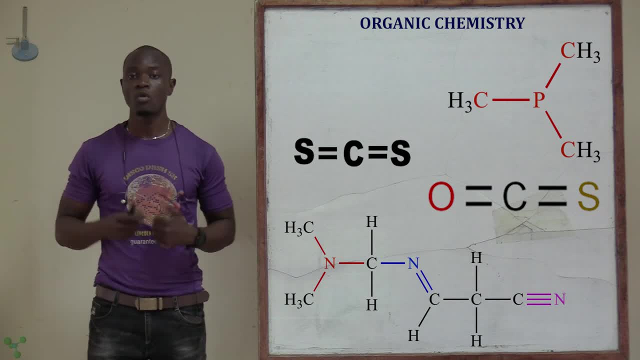 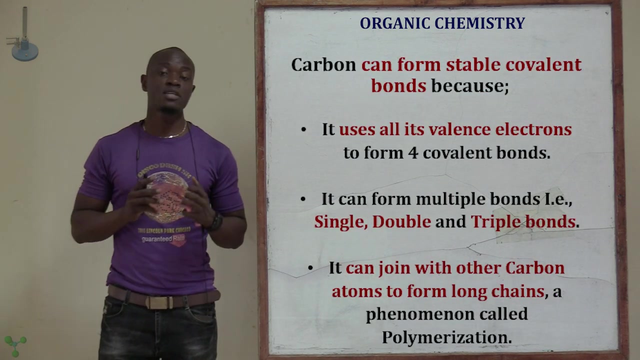 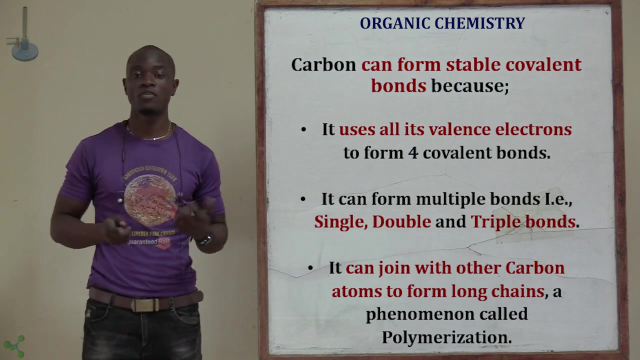 the carbon can bond with hydrogen, or the carbon can bond with other, with the other atoms that are in the periodic table. so why is it that the carbon atom is able to to form different types of bonds? so the first reason: we see that the carbon atom uses all four valence electrons in order to form the covalent bond. so it uses all four. 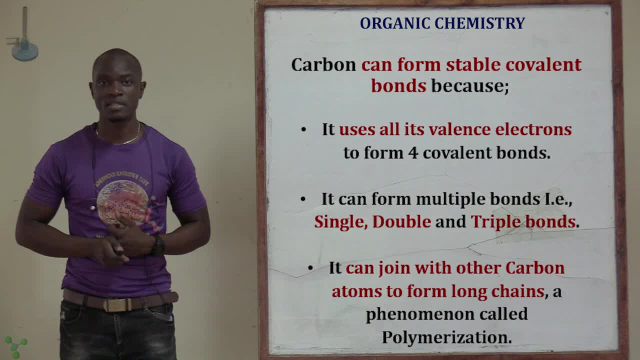 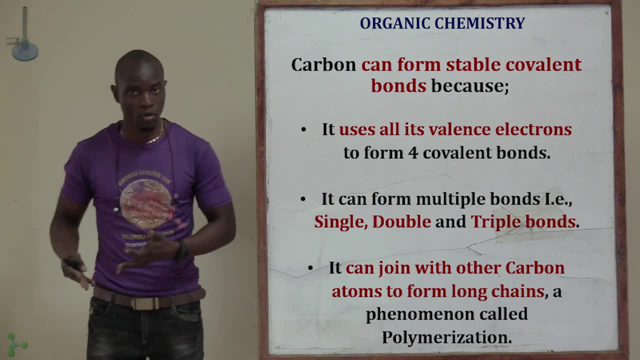 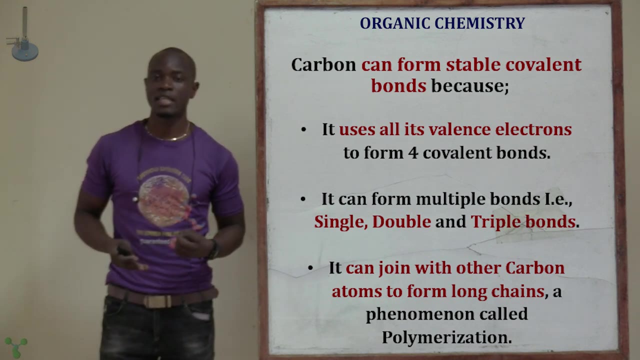 valence electrons in order to be able to form the bonds that there is also. apart from that, you see that the carbon atom is able to form a single bond, is able to form a double bond, is able to form a triple bond with other carbon atoms or with other elements as large, like, for example. you see, 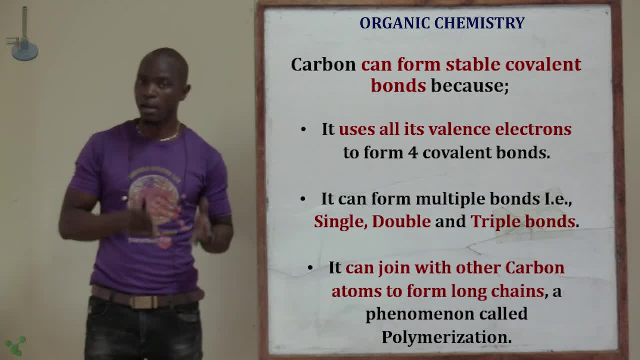 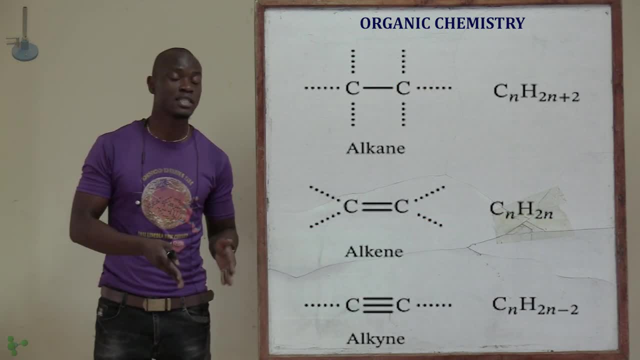 that the carbon atom can be able to form a single bond between carbon and other carbon atoms, and it can be able to form a single bond between carbon and other carbon atoms, whereby, in the hydrocarbon families, you are going to see that this family will be called the alkynes. 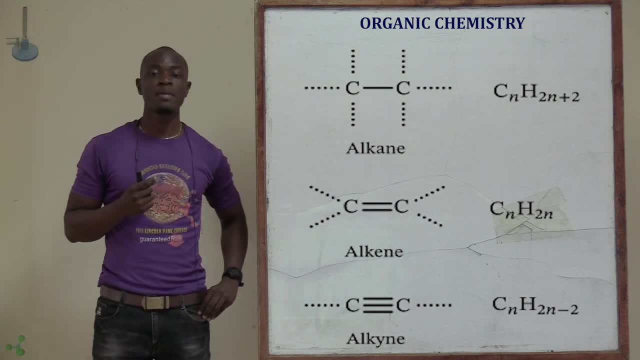 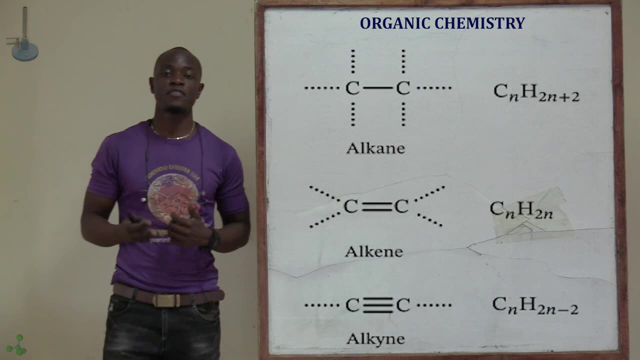 apart from that, you see that the carbon atom can also be able to form a double bond between other carbon atoms or between other atoms in the periodic table and this family which have double bond between the carbon atoms. we are going to look at it, it's called the alkynes. and then, finally, we have 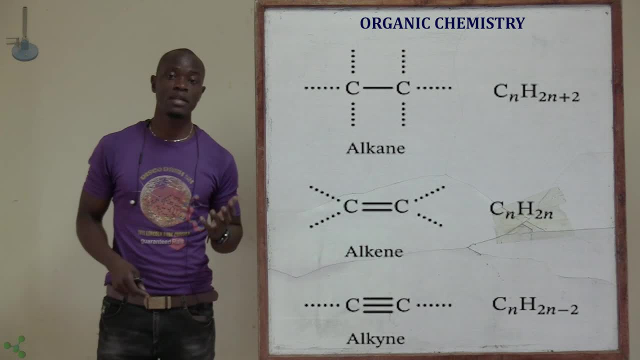 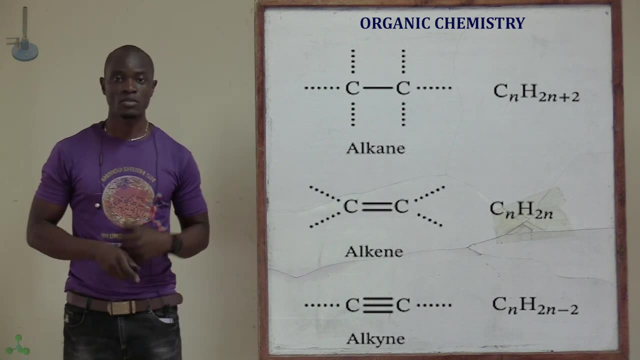 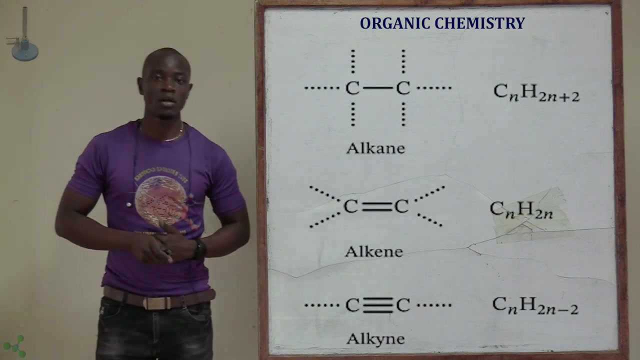 the alkynes. for the alkynes, as you can see, alkynes from the family whereby the carbon atom is bonded using three covalent bonds to other carbon atoms or to other elements. so a single bond is called an alkene, a double bond, the family, is called an alkene. and a triple bond, the family will be called an. 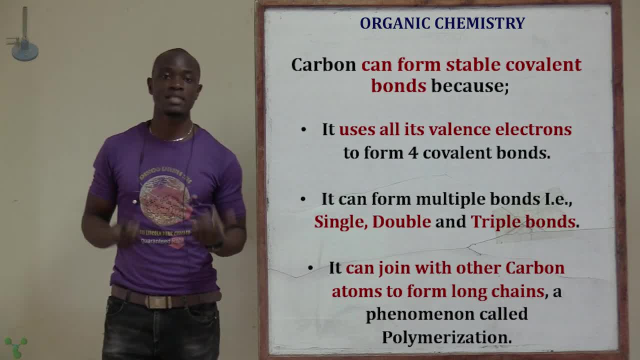 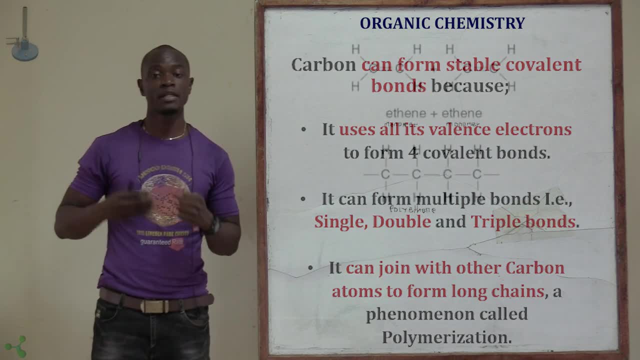 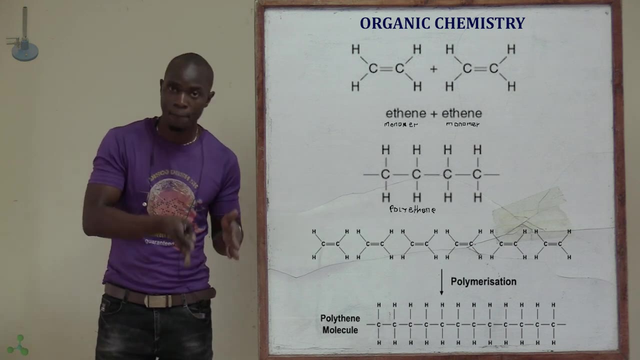 alkynes. so, apart from that, the third reason, we can say that the carbon atom is able to join with other different carbon atoms to law, to form very long chains, a phenomenon which is called polymerization. so the different monomers, so the different monomers of carbon, are the different. 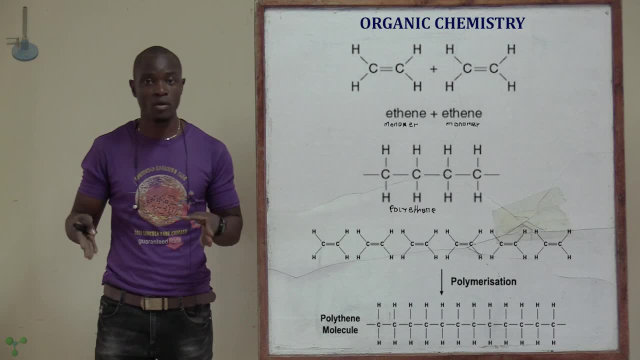 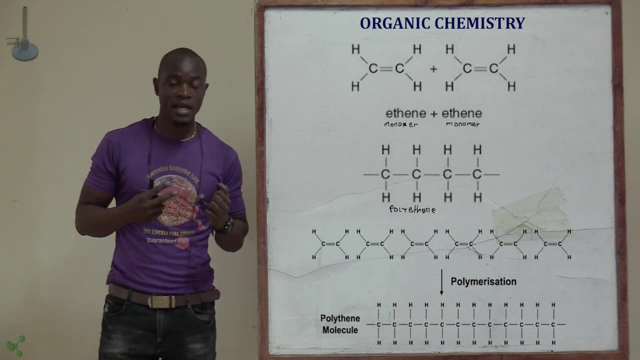 carbon can be able to react with other different monomers of carbon to form a very long chain, which is referred to as a polymer. now, the process by which monomers react to form a polymer, that process will see that it is called a polymerization reaction. so this polymerization reaction we're 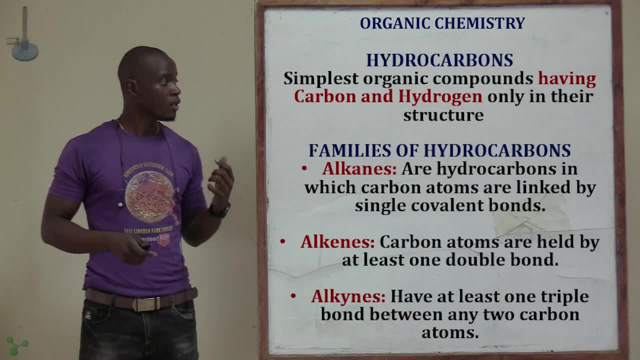 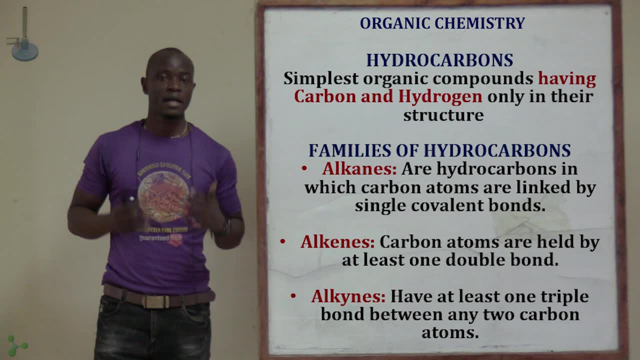 going to look at it in the upcoming subtopics. so, apart from that, let's now look at uh hydrocarbons and see what are hydrocarbons. so mainly hydrocarbons. as we studied, we introduced hydrocarbons in form one and we saw that the hydrocarbons, so this mainly. 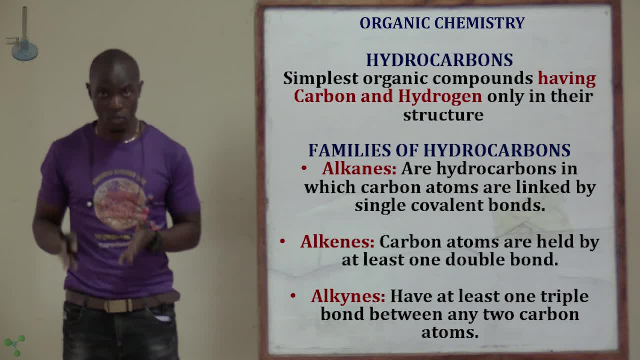 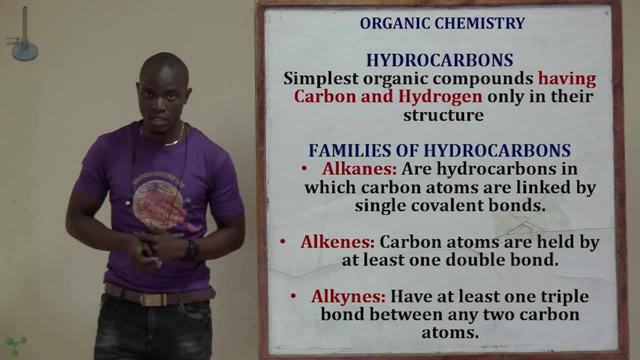 comprises of carbon bonded to hydrogen only. so if carbon is bonded to hydrogen, only that compound is referred to as the hydrocarbon. so this, mainly the hydrocarbon- mainly forms a compound whereby carbon is bonded to hydrogen, so that component is called a hydrocarbon. we see that the hydrocarbon 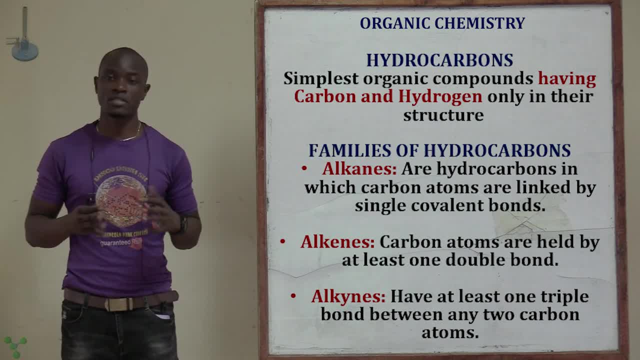 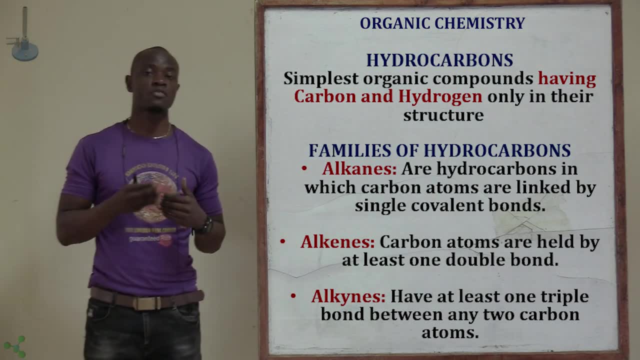 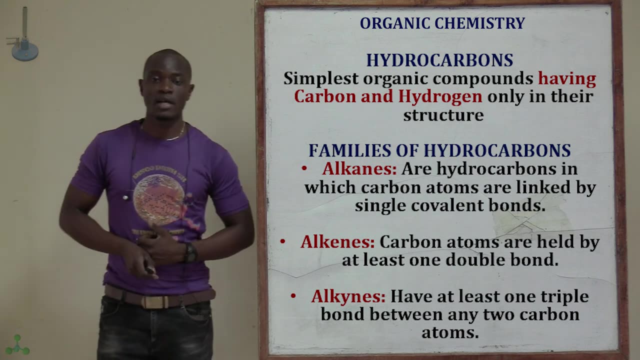 are the simplest organic compounds that we have, Because they mainly comprise of only carbon and hydrogen in that compound. So that is that It only comprises of hydrogen and carbon in that compound. So that compound is referred to as the hydrocarbon. So, apart from that, let's now look at the main. 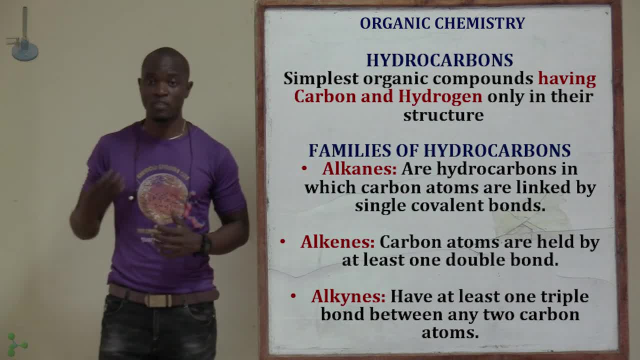 groups or the families of hydrocarbons, Because we have different families of hydrocarbons, example, like for the ones that we have just introduced, So they can be called families or they can be called the main groups. So, in example, if you have been asked, what are the main groups, 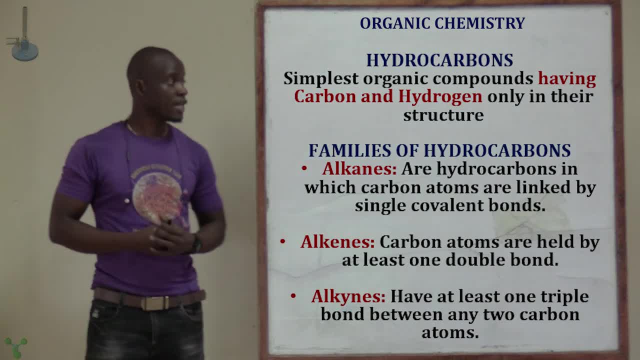 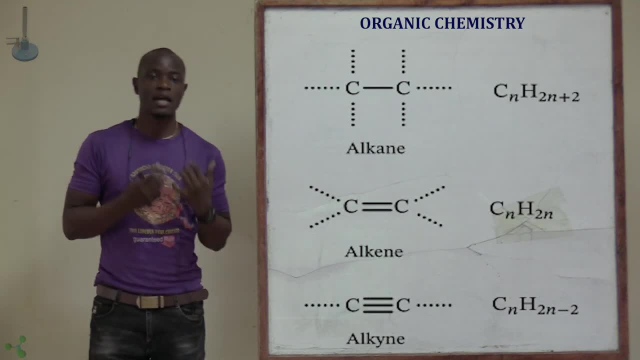 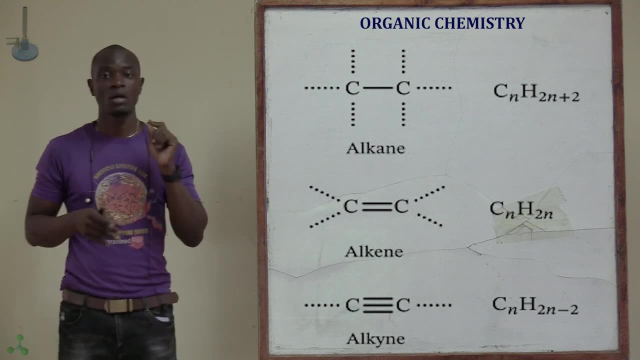 or what are the main families, or the families of hydrocarbons. So they include, as you can see, so they include the alkenes, like whereby we say that alkenes So these are hydrocarbons, whereby the carbon is bonded to one covalent bond, So the carbon is only bonded to one covalent bond. 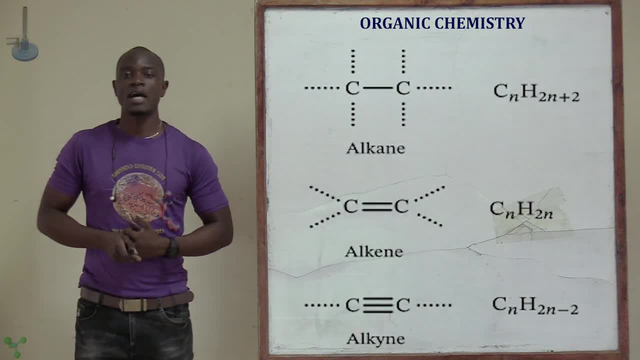 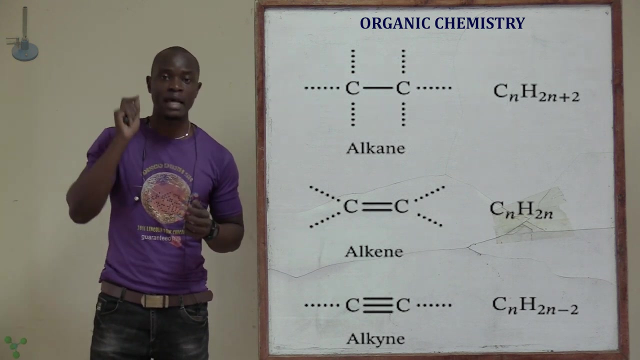 So, apart from that, the other family, we have the alkenes. So what are the alkenes So like? for the alkenes, we see that alkenes, this is a family whereby carbon atom is bonded to two covalent bonds. So in this structure of the alkenes there is at least a double bond in the 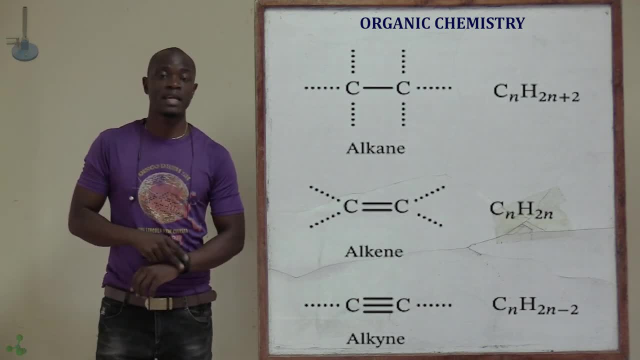 structure. So apart from that, the third family we have, we have the last family which is now referred to as the alkynes. So the alkynes, this is the hydrocarbon family whereby the carbon atom is bonded to three covalent bonds. So at least in the structure of the alkenes there is at least a 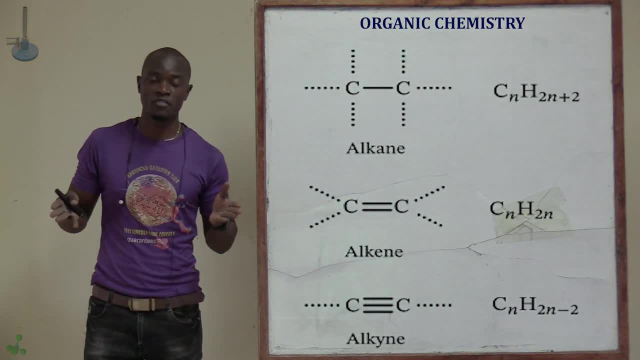 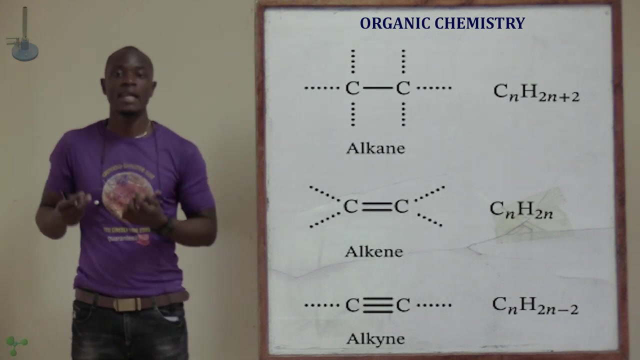 triple bond in this structure, like at least in the molecule of this or in the structure of the alkyne. So you're going to see at least a triple bond. So in the molecule if you see a triple bond you'll know automatically this is an alkyne because it has three covalent bonds in the structure. 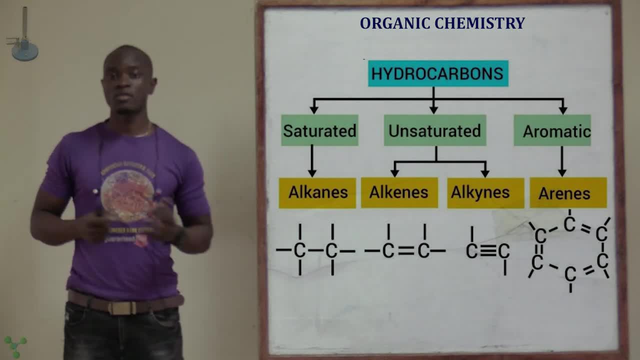 So, apart from that, let's continue to another definition of terms, whereby let's also define between saturated and unsaturated hydrocarbons, as well as the chromatic hydrocarbons. So what are saturated hydrocarbons? So, for the saturated hydrocarbons, 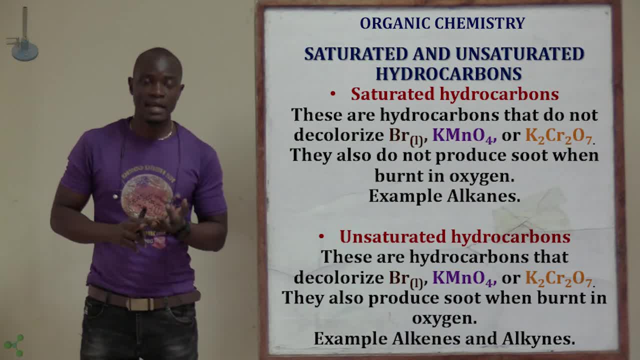 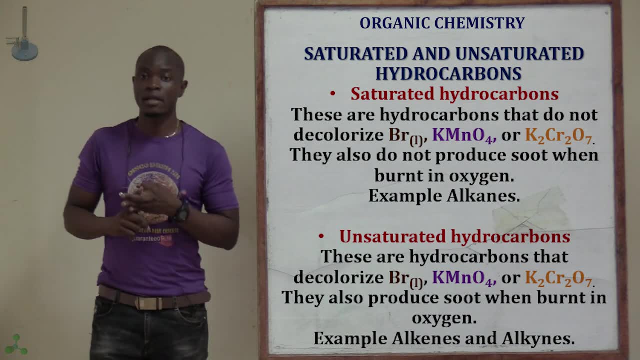 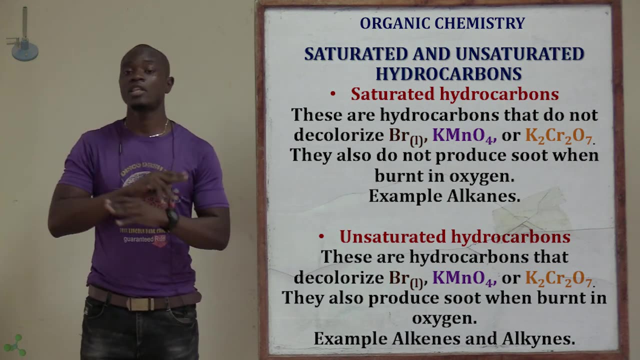 these are hydrocarbons which cannot discolorize bromine water. They cannot discolorize potassium permanganate, They cannot discolorize potassium dichromate And as well the saturated hydrocarbons. when burnt they do not produce soot, So they do not have any soot, They don't produce soot. 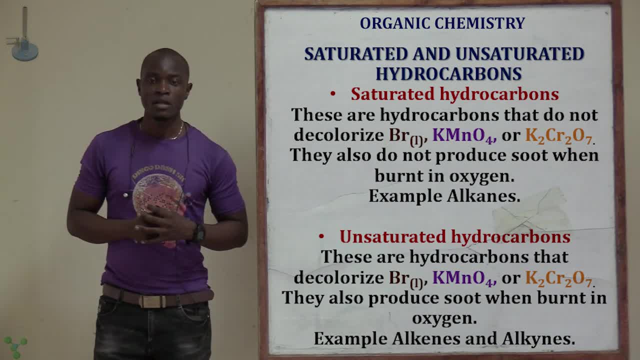 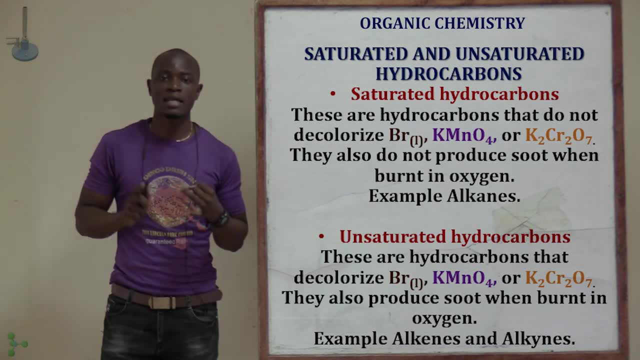 Example: you see the kerosene. So they do not produce soot. So these types of hydrocarbons, which cannot discolorize potassium permanganate, they cannot discolorize bromine water, They cannot discolorize potassium dichromate. 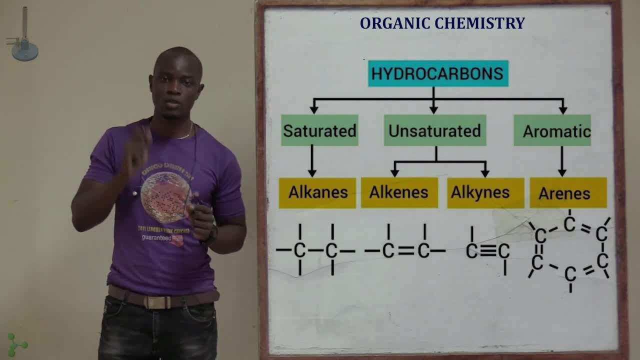 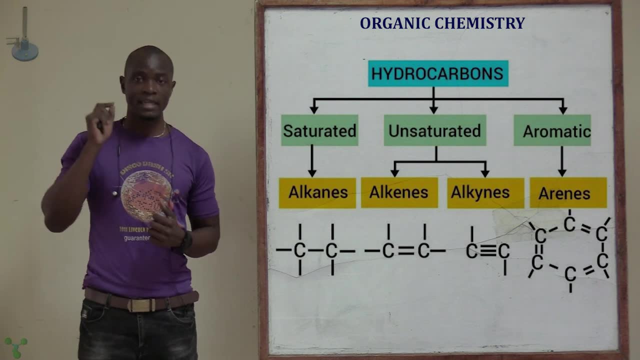 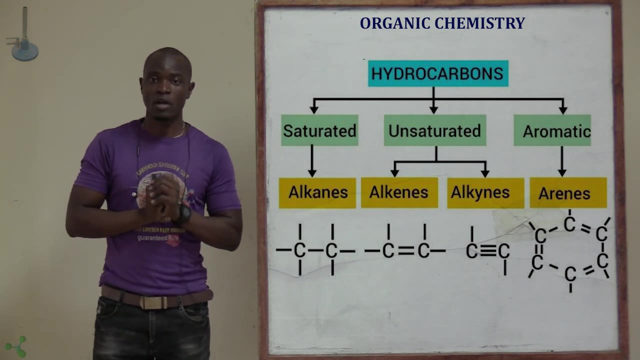 And when burnt they don't produce soot. So these hydrocarbons, they are referred to as the saturated hydrocarbons. Example of saturated hydrocarbons: in the three families we have the alkenes. So all the members of the alkenes, all the members, they are saturated hydrocarbons. 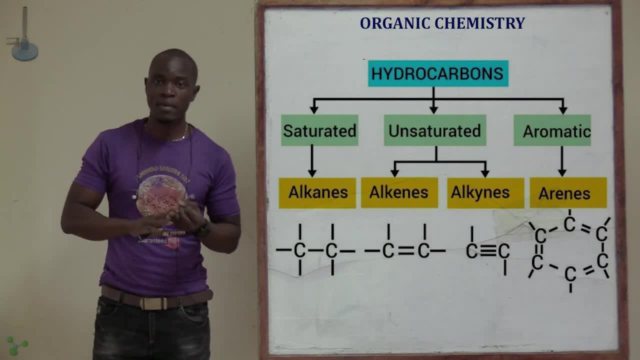 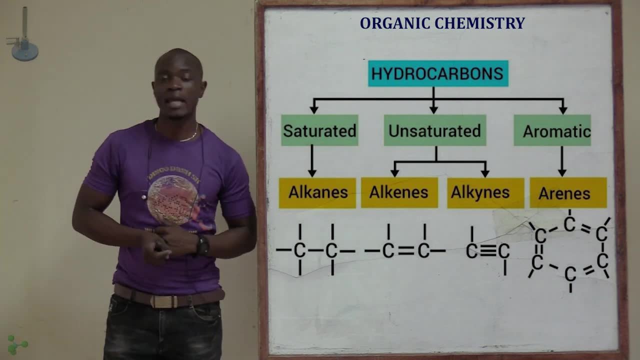 Meaning that they do not produce soot when burnt. Potassium, permanganate, dichromate, bromine water do not discolorize, So these are saturated hydrocarbons. Remember, they only comprise of the alkenes in the family of hydrocarbons. So, apart from that, we have now the, we have the. 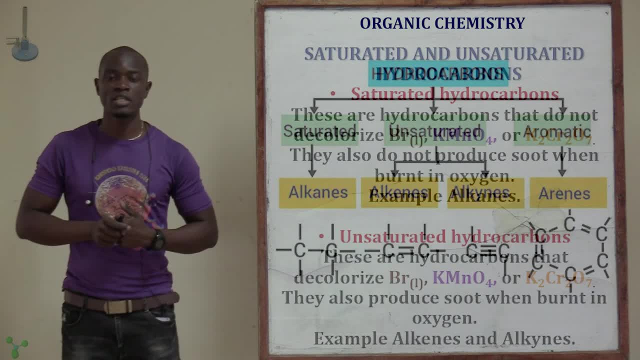 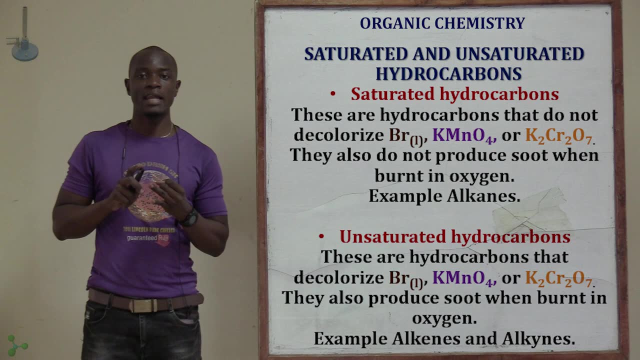 second one, which is the unsaturated hydrocarbons. And for the unsaturated hydrocarbons, remember, the unsaturated hydrocarbons mainly comprise of the alkenes and the alkynes, So it comprises of those two which are the unsaturated hydrocarbons. And for the unsaturated hydrocarbons, remember, 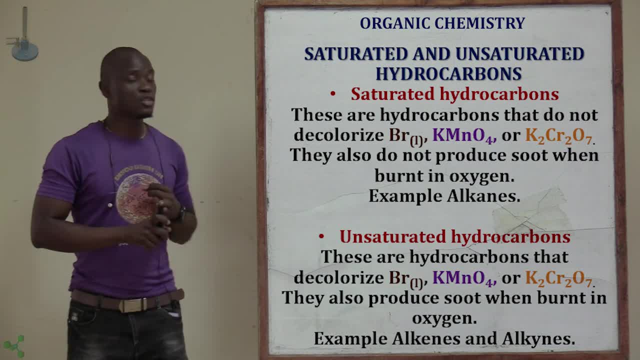 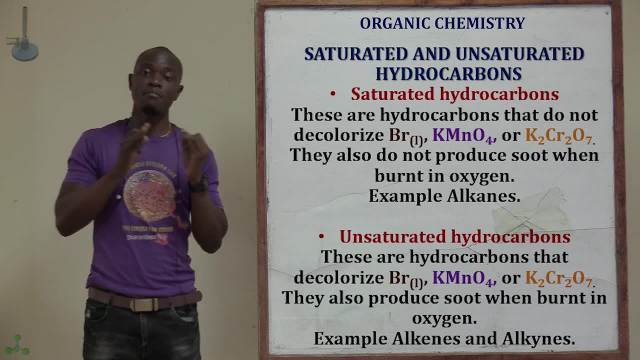 which are the alkenes and the alkynes. So for the unsaturated hydrocarbons, we see that they can be able to discolorize bromine water, They are able to discolorize potassium permanganate, They are able to discolorize potassium dichromate And as well when they are burnt in the atmosphere. 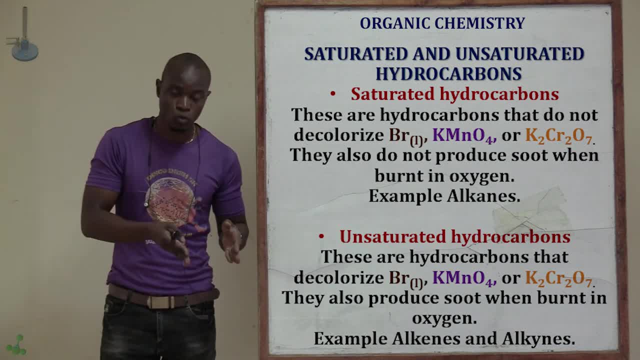 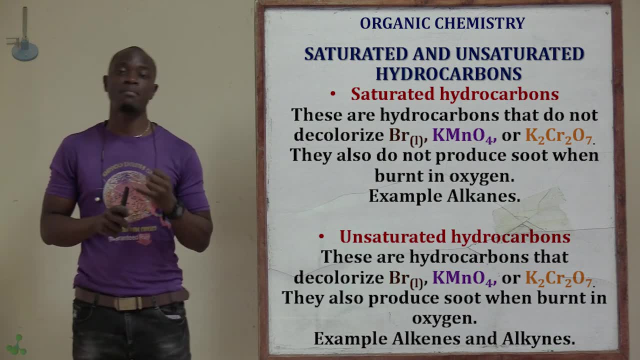 they produce soot. Alkenes produce less soot, but alkynes produce the most, The most amount of soot. So, in short, the unsaturated hydrocarbons. they can be able to discolorize- bromine, water, potassium permanganate, potassium dichromate, And as well when burnt. 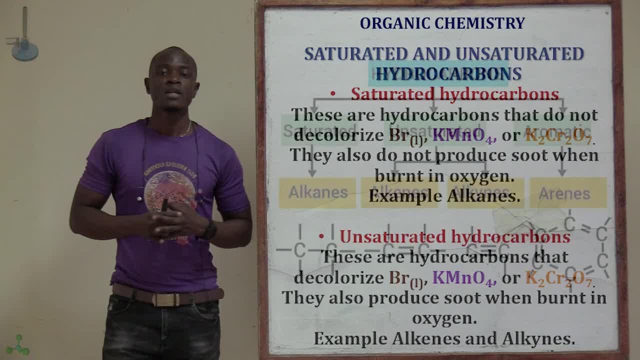 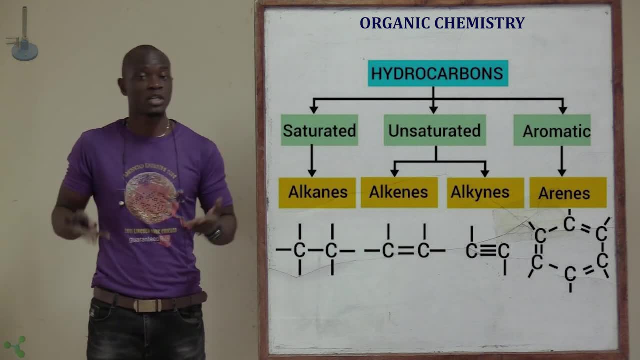 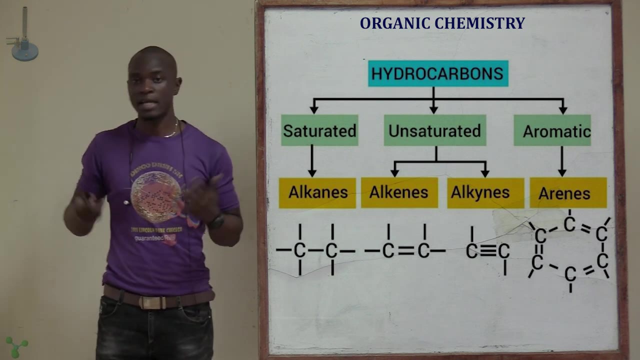 they produce a lot of, they produce a lot of soot. So in the families, in the three families, we see that the families of the members in the family which belong to unsaturated hydrocarbons, we have the alkenes and we also have the alkynes, So they all belong to the unsaturated hydrocarbons. 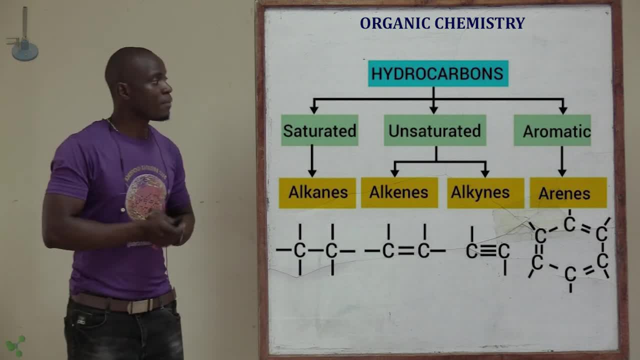 for the reasons that we have mentioned. So for the unsaturated hydrocarbons, we have the alkenes and we велp of both alkenes and alkanes. All the answers have been already explained by the sessions that we have just stated. So, apart from that, you can see that we have 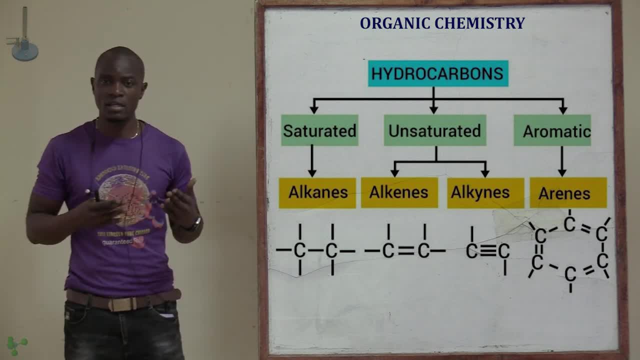 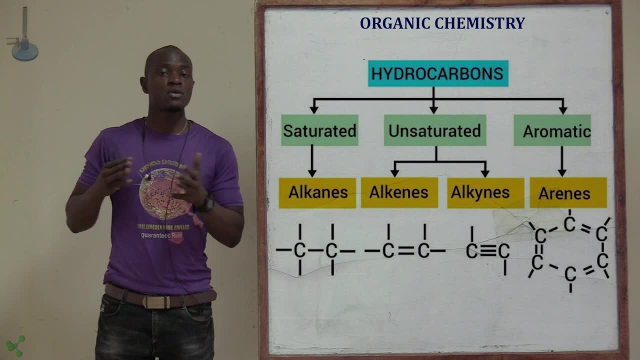 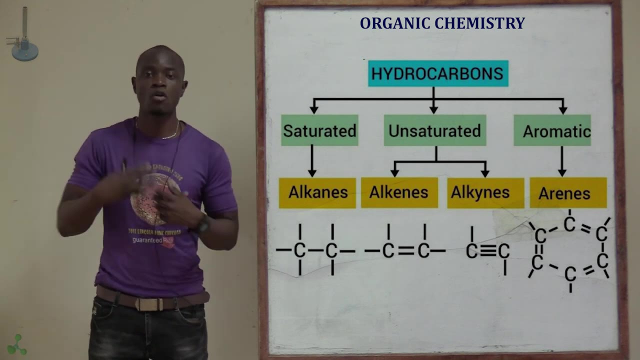 the aromatic hydrocarbons, whereby, for the aromatic hydrocarbons, this mainly comprises of the benzene rings. So the benzene rings, mostly they appear in the aromatic hydrocarbon. So why is it that they appear in the aromatic hydrocarbon is because most of these structures have a sweet scent. Most of these structures they have. 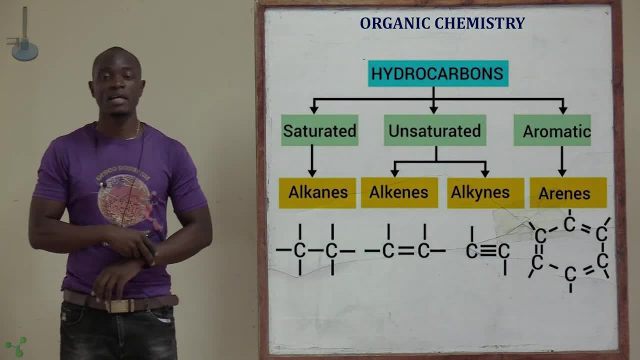 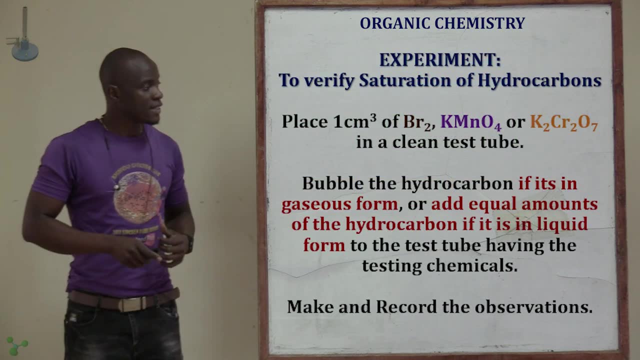 so they can have different types of smells and that's why they fall under the aromatic hydrocarbons. so, apart from that, let's look at an experiment by which you can be able to determine or be able to distinguish between saturated and unsaturated hydrocarbons. so in the experiment you can use different test. 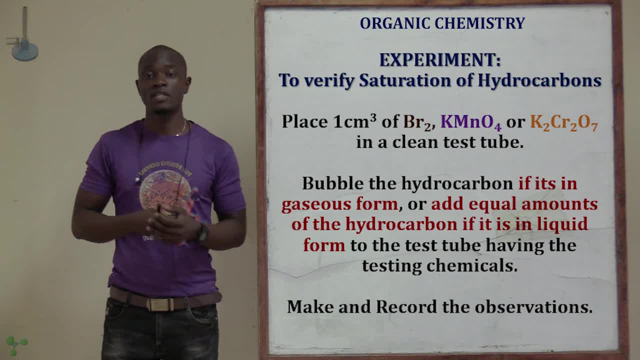 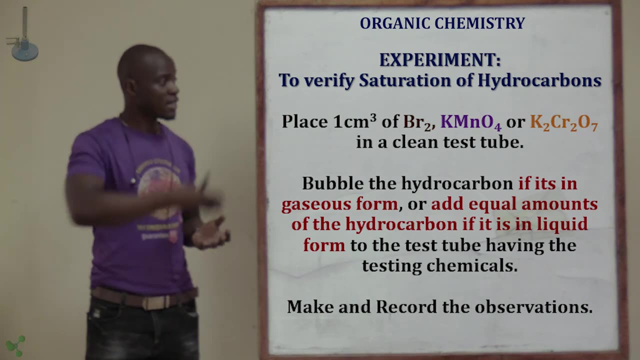 tubes we can use gaseous hydrocarbons or we can use the liquid hydrocarbons. so for the experiment heading, we can say the heading to verify saturated and unsaturated hydrocarbons. so that is the heading of the experiment. then after that you have the apparatus, which will be listed, and then we go to procedure. so 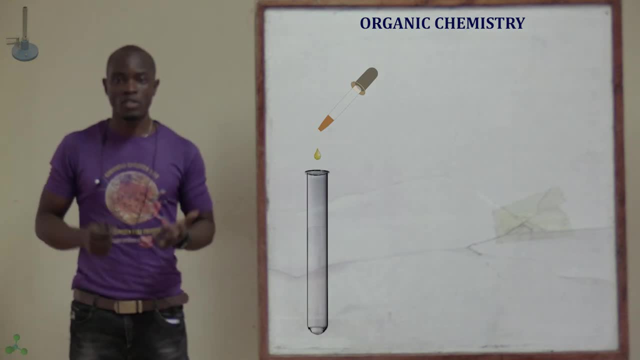 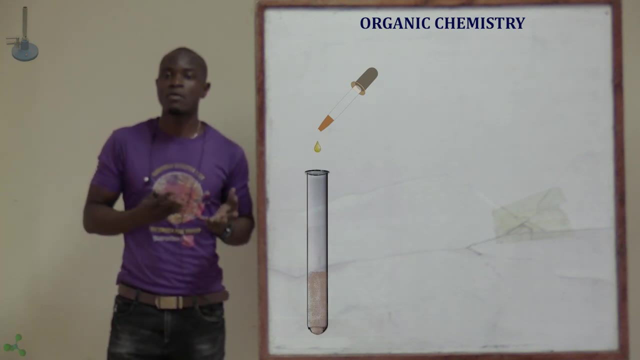 for the procedure. we can say: add three to four drops of bromine water to a clean test tube. so rather, let's say: at least add one centimeters cubed. add one centimeters cubed of brown bromine water in a clean test tube. so rather, let's say, at least add one centimeters cubed, add one. 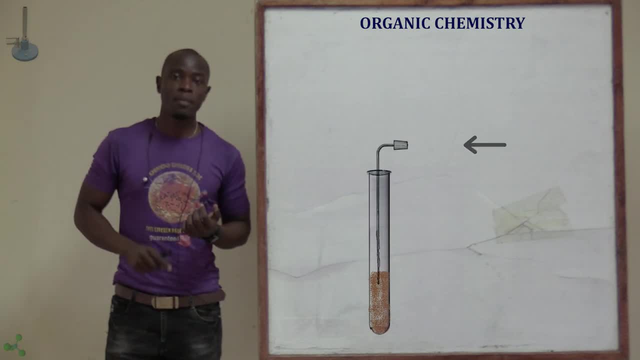 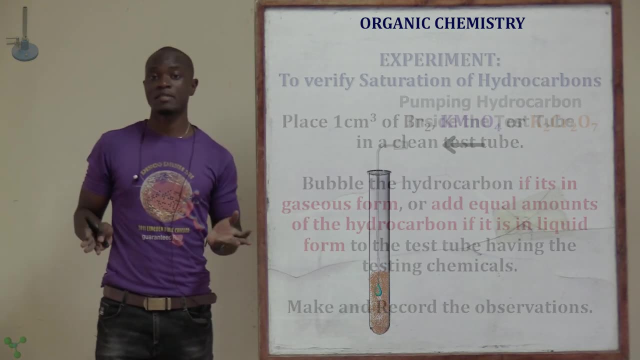 centimeters cubed of brown bromine water in a clean test tube. so after that we can say: bubble the hydrocarbon inside bromine water and then make observations. so that is just the experiment. so add one centimeters cubed of bromine water in a. 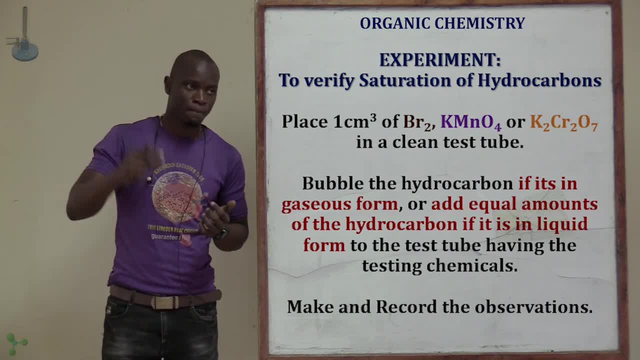 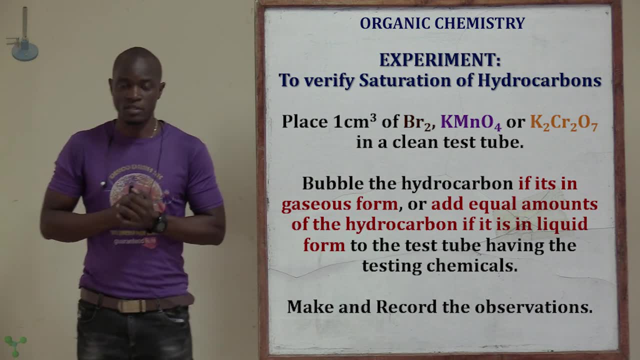 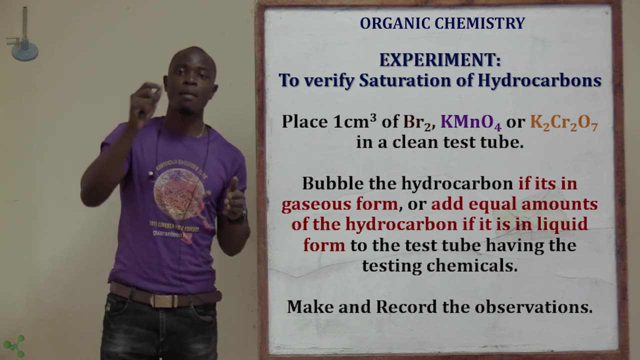 clean test tube and then bubble the hydrocarbon inside the bromine contained inside the test tube and then finally make observations. so that is, if we are using gaseous hydrocarbons. so if you are using a gaseous hydrocarbon, we are going to bubble the gas inside the bromine water. 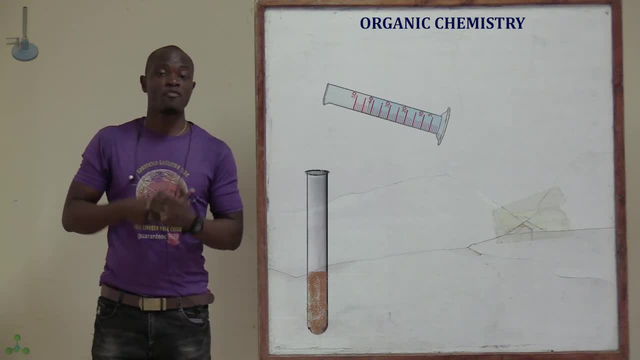 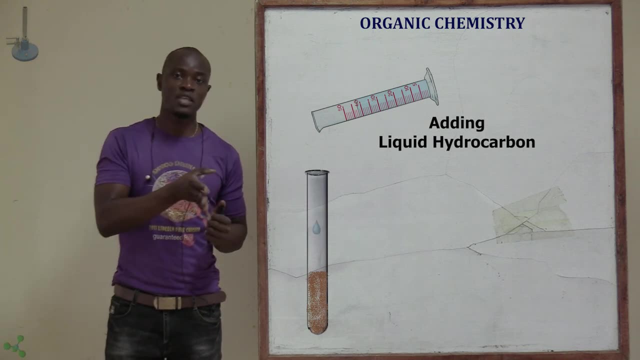 but if we are using liquid hydrocarbon, like for example we have pentane, hexane, heptane octane, nonane, decane, if you are using that, we are going to add at least half amount of the bromine water that was added, or equal amount. so if you are, 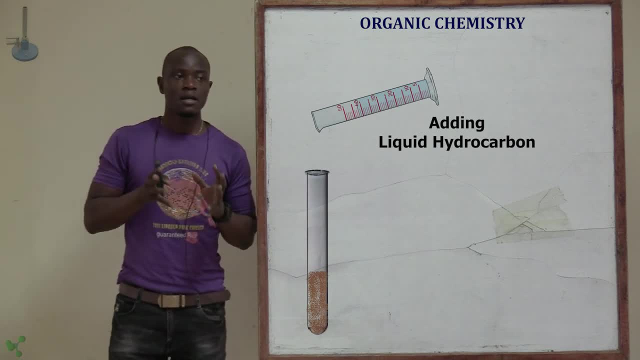 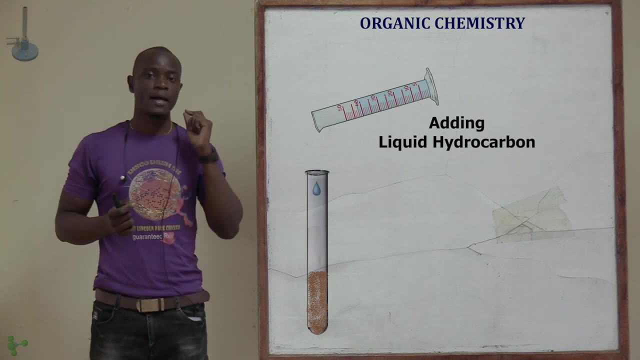 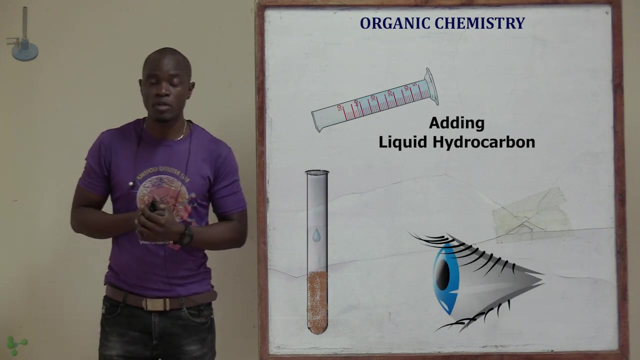 using a liquid hydrocarbon. we'll say like: add one centimeters cubed of bromine water inside a clean test tube. so after that you can say: then add one centimeters cubed of the hydrocarbon liquid in the test tube having bromine water and make observations. and then finally you're going to make observation. 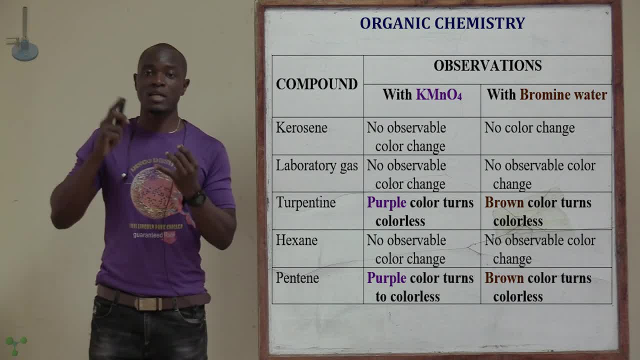 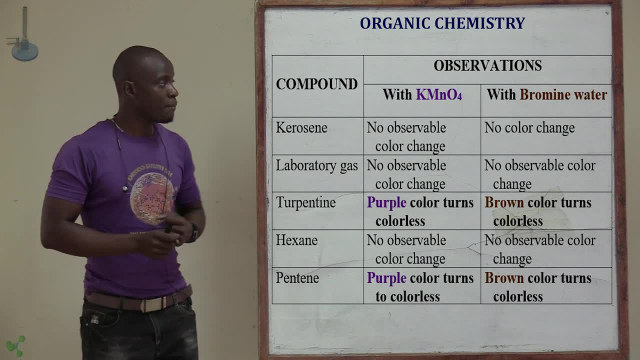 so the same same experiment you can repeat using potassium permanganate or potassium dichromate in place of the bromine water. so what are the observations make made? let's compare between potassium permanganate and bromine water to see the observation, using the different compounds that you. 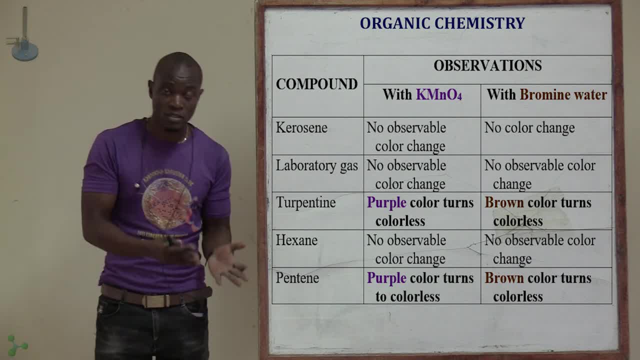 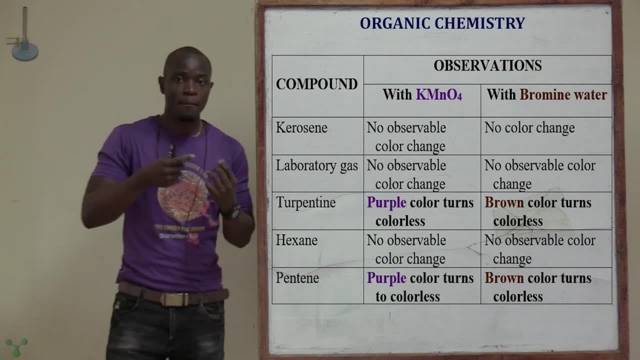 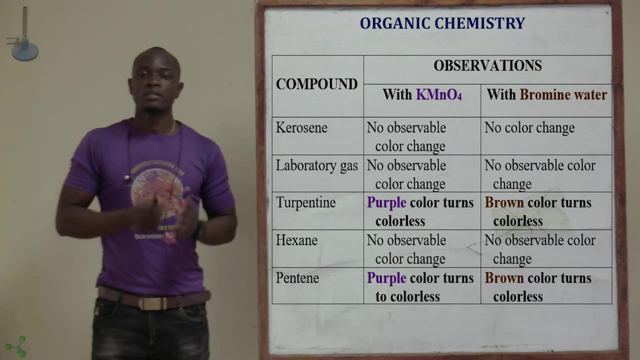 have. so the first compound, let's test the first compound that we know. let's test kerosene. so you take kerosene and then we bubble kerosene inside potassium permanganate and then we also bubble the kerosene inside bromine water. so if we 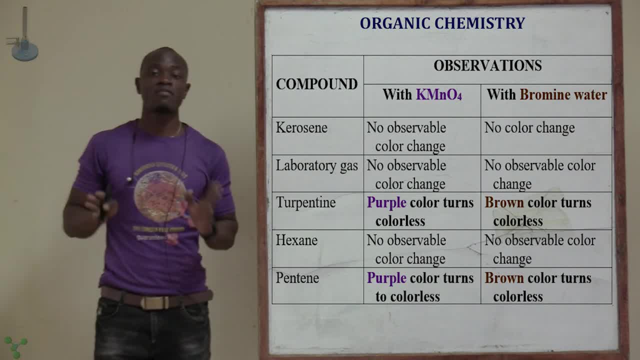 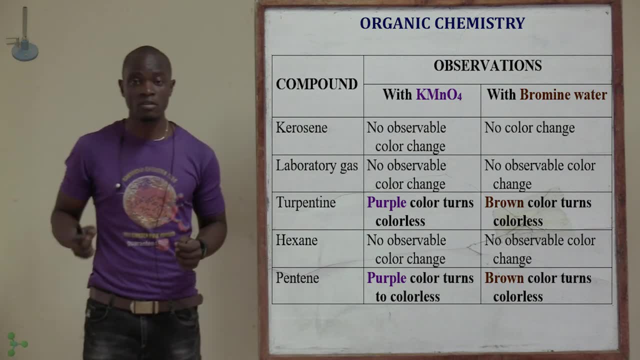 mix the kerosene with potassium permanganate, there'll be no observable color change. if we mix it with bromine water, there is no observable color change. it means that kerosene falls under the family of family of alkanes, because kerosene is unable to discolorize. 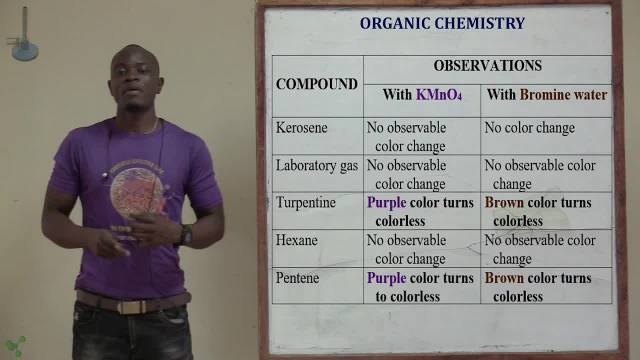 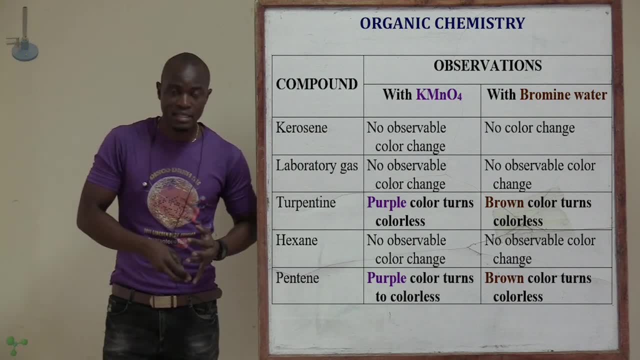 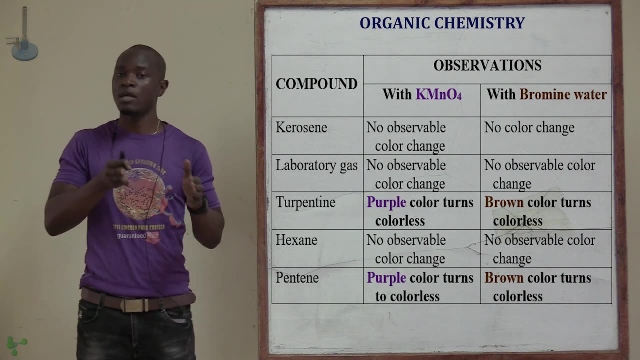 potassium permanganate or bromine water. so, apart from that, you can use another compound, which is now the laboratory gas. laboratory gas, it can be methane gas, it can be butane gas, just from the word methane ending with a n e and butane ending with the word a n e. it means that these are 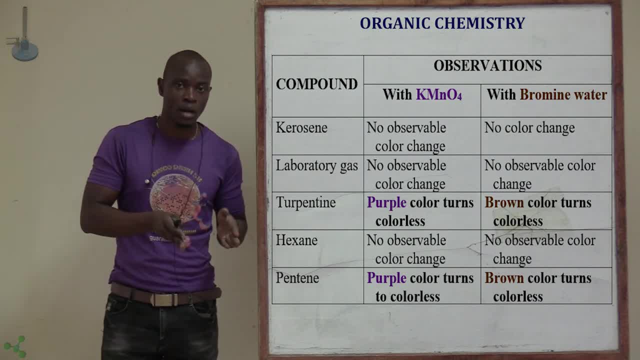 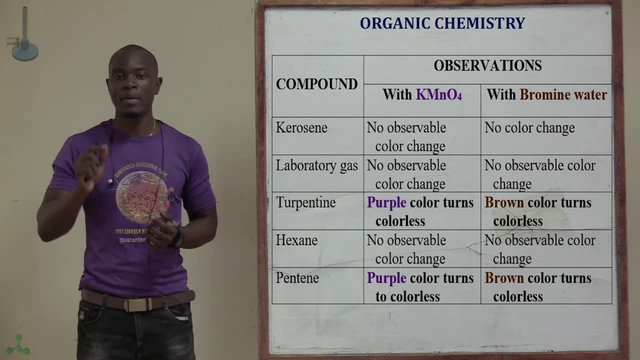 alkenes. since these are alkanes, alkenes are unsaturated hydrocarbons, so we expect there is no color change that is going to be observed. so if we bubble the laboratory gas inside potassium permanganate, no observable change will be will take place, and also in bromine water. 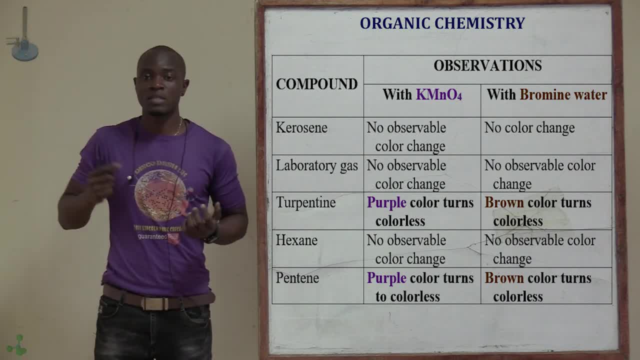 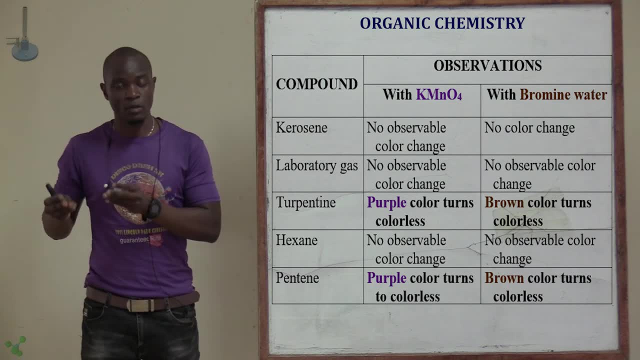 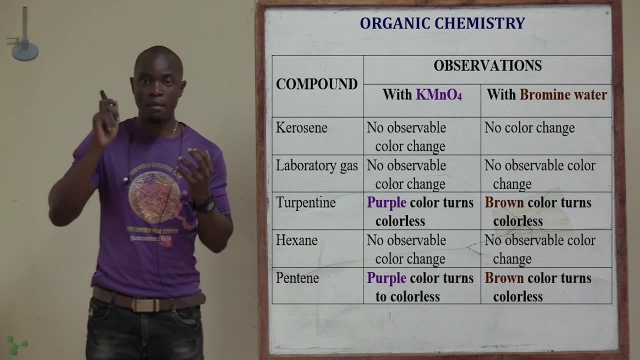 no observable change is going to take place. so why is it that no observable change will take place? it's because laboratory gas methane and butane. so these these gases are alkenes, and they say that alkanes are saturated hydrocarbons, So they don't discolorize bromine, water or potassium permanganate. 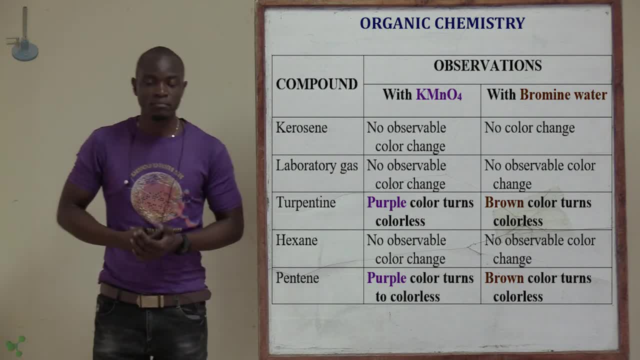 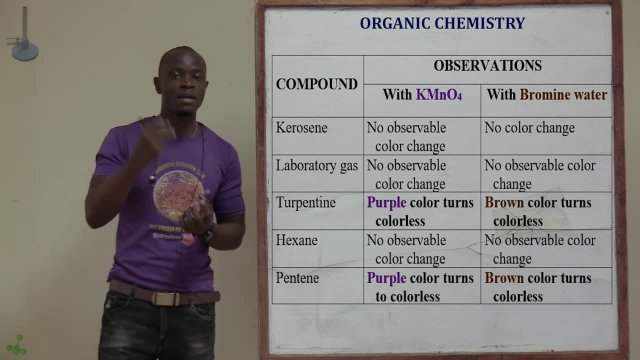 So, apart from that, we can use also the turpentine, whereby the turpentine is like a liquid, The oil that is used in making the roads, that very black oil. the black oil that is used in making roads is the one which is called turpentine. 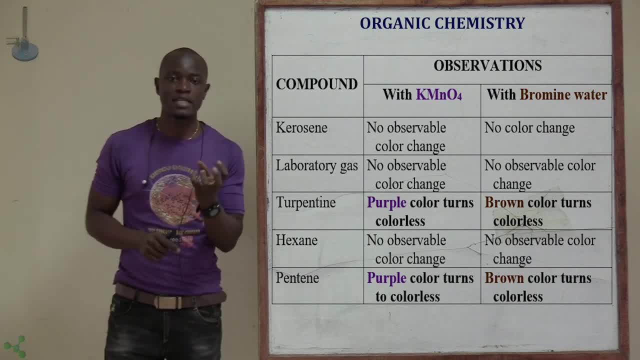 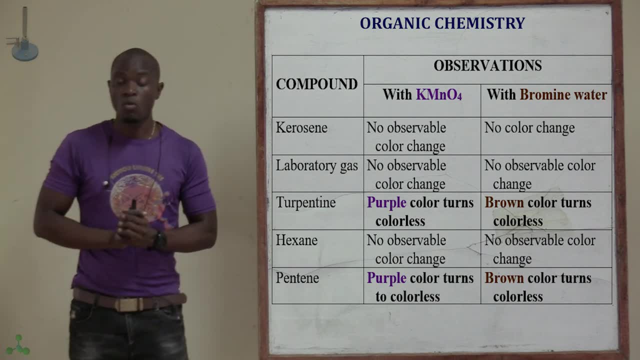 So let's use turpentine. So if we add the turpentine in potassium permanganate, so we'll see that it is going to discolorize the potassium permanganate. Why is this so? It's because turpentine is an unsaturated 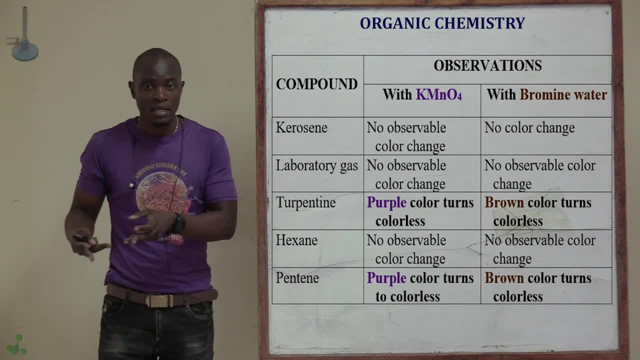 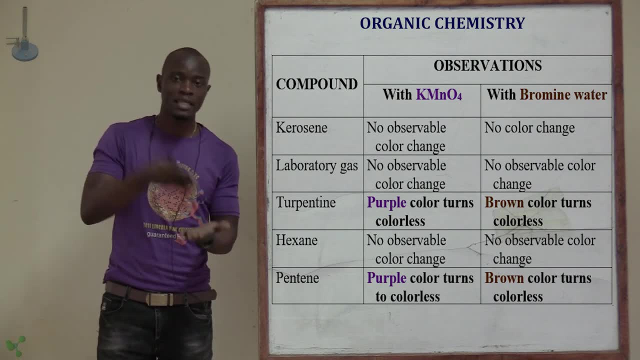 So, since it has discolorized the potassium permanganate. therefore, the conclusions made is that turpentine is an unsaturated hydrocarbon, meaning that it can fall between alkene or an alkyne. So the same same, the same same: the turpentine. 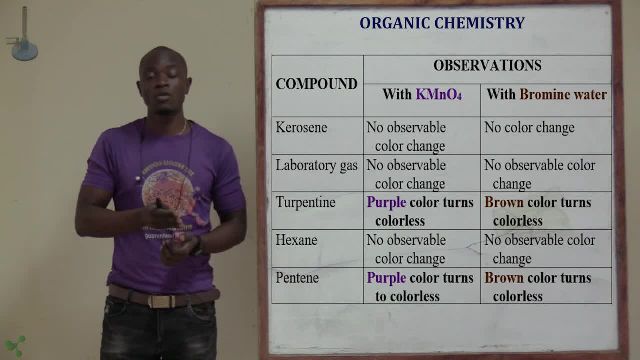 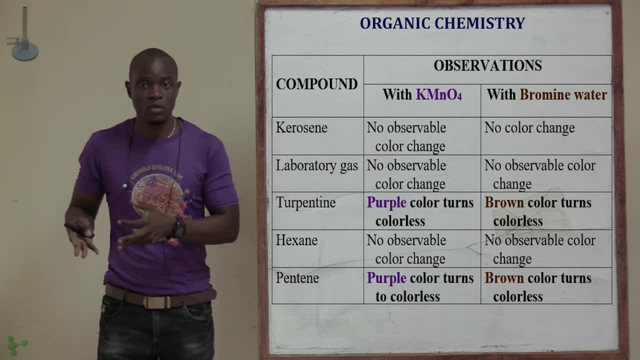 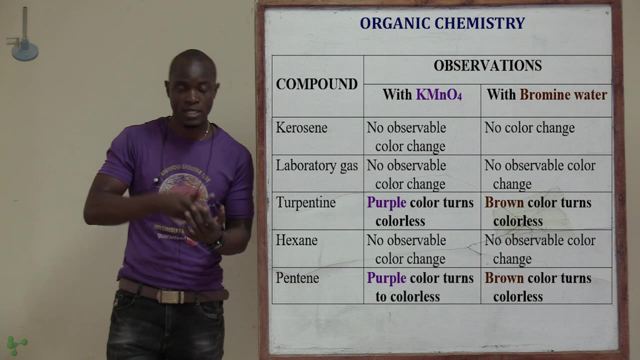 We add it, We add it to bromine water. So if we add it to bromine water, it is going to discolorize the bromine water. So what are the results we are going to see? So if it has discolorized bromine water, therefore, results will say that turpentine is an unsaturated hydrocarbon because it has discolorized bromine water and potassium permanganate. 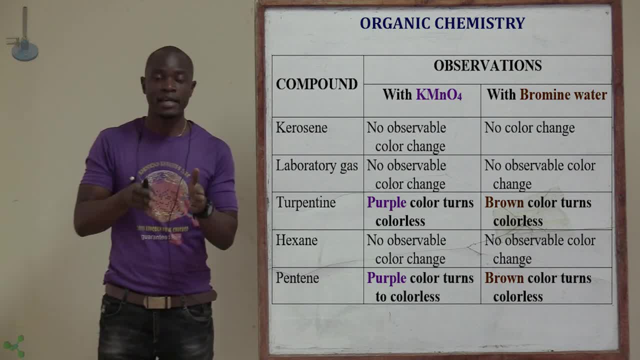 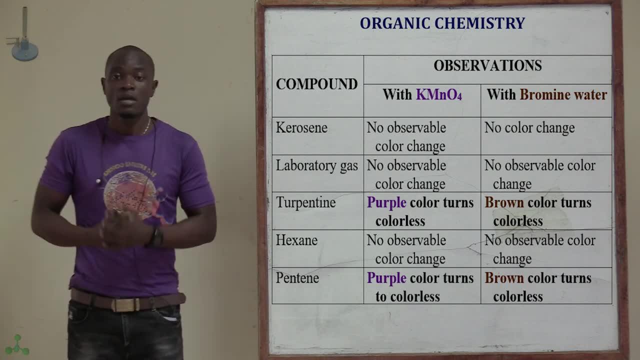 Then the next one is hexane. Hexane, just as the word ends A-N-E, it means that this is an alkene. So if it's an alkene, alkenes are saturated hydrocarbon. So if they are saturated hydrocarbons, it will mean that hexane will not discolorize potassium permanganate or bromine water, because it falls under the family of alkenes. 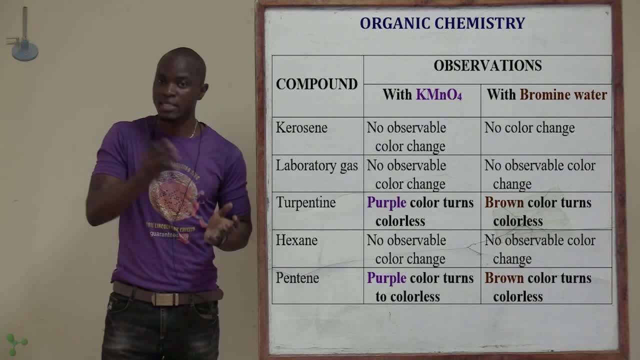 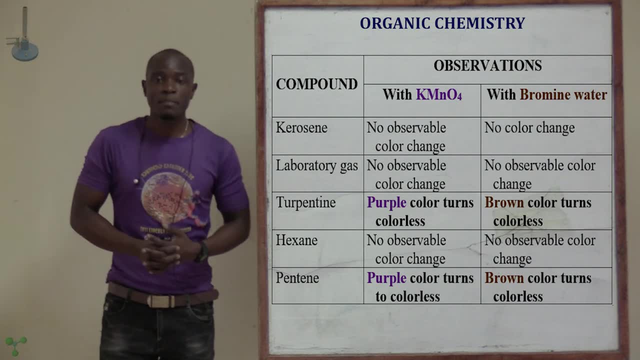 Alkenes are saturated hydrocarbons. They don't discolorize potassium permanganate, bromine water or potassium dichromate. After that we have the next one is pentene. What happens when we dissolve pentene in potassium permanganate or bromine water? 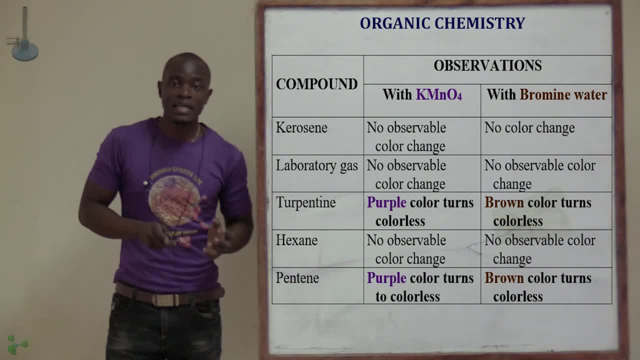 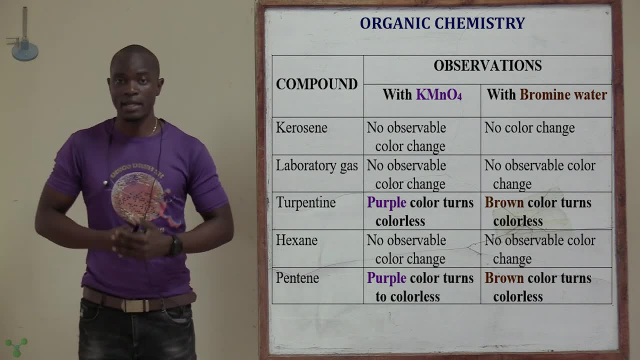 So what will happen is that the potassium permanganate is going To discolorize. The bromine water also is going to discolorize. So why is it that it is going to discolorize Now? it will discolorize because pentene is an alkene. 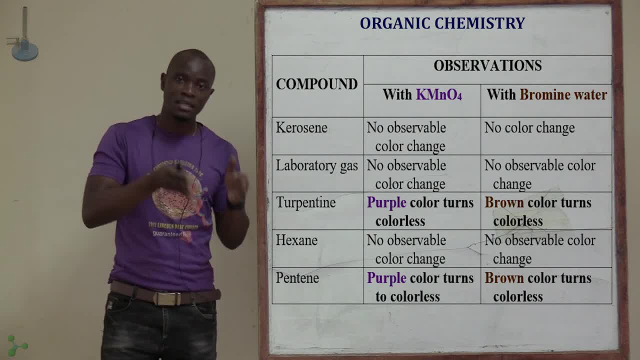 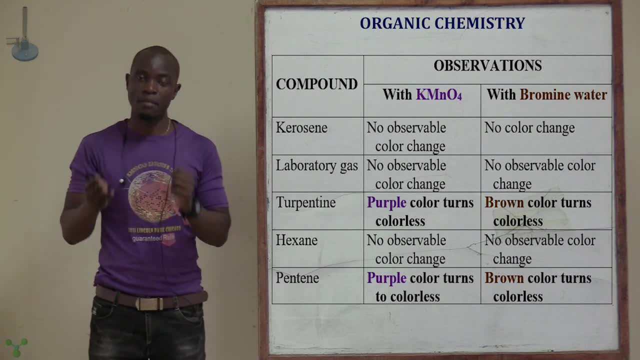 Since pentene is an alkene- remember we say that all alkenes are unsaturated hydrocarbons. So since it is an alkene, it is going to discolorize the potassium permanganate and the bromine water because they are unsaturated hydrocarbons. 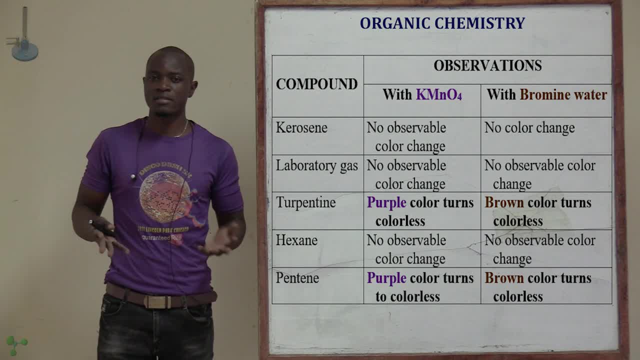 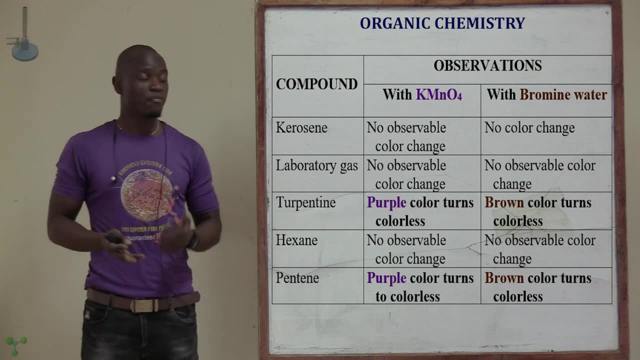 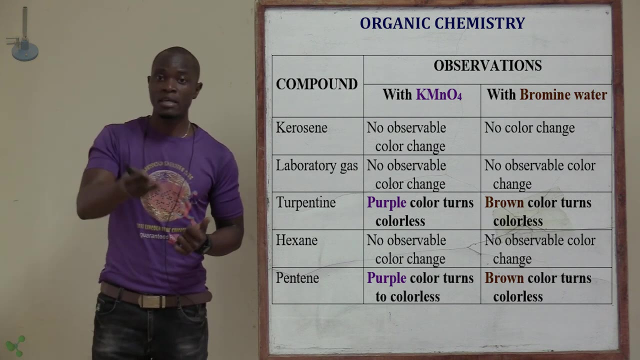 So that is that in as far as the saturated, unsaturated hydrocarbon is concerned. So that is that You can be asked a question in an exam. You have been given pentene or the same question, So explain which hydrocarbons are, saturated or unsaturated. being given potassium permanganate? 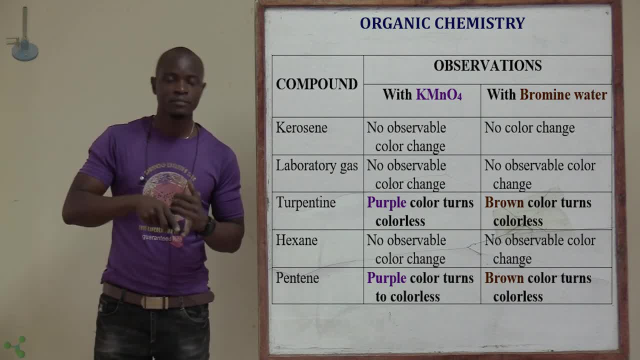 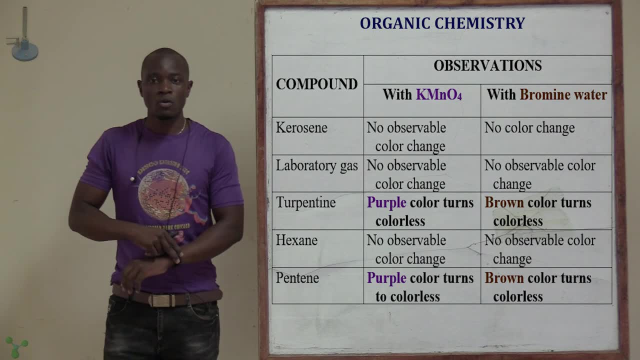 So you are just going to look at the experiment. If you see it's an alkene unsaturated, it's going to discolorize. If you see it's an alkene saturated, no discolorization. So what happens?